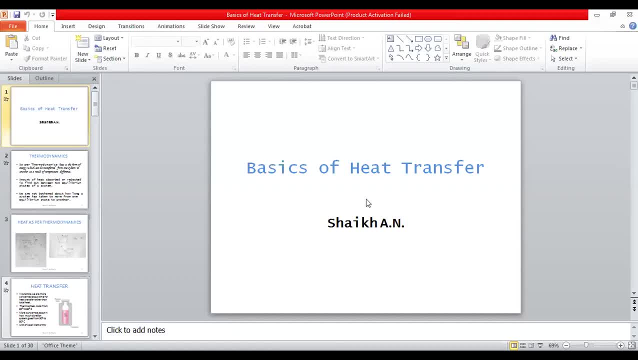 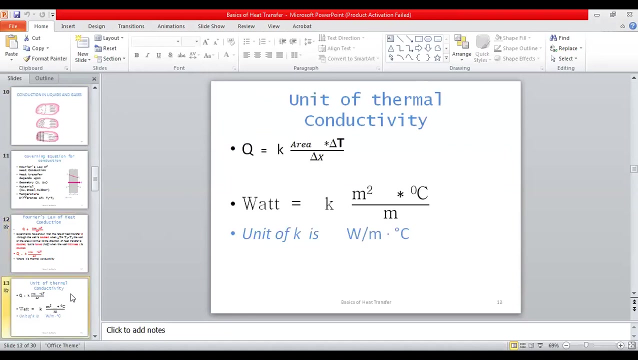 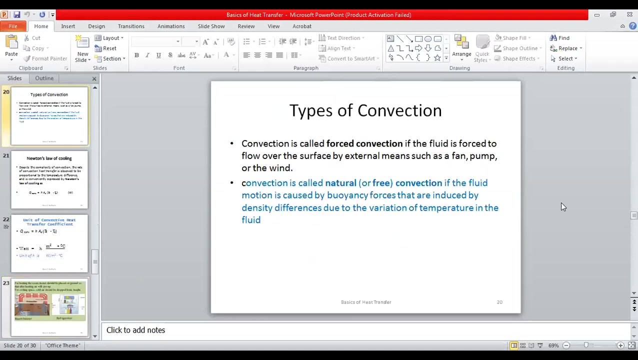 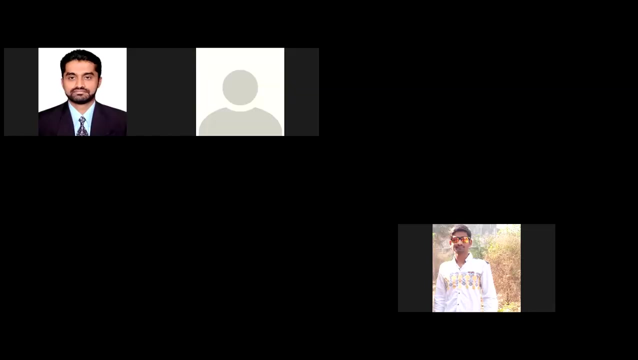 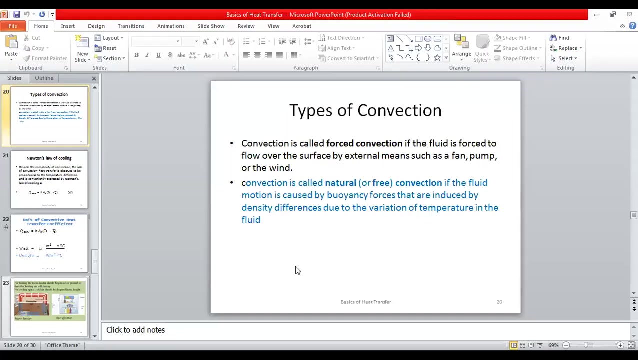 Thank you, Thank you. Don't play with screen. Don't touch the screen. Don't touch the screen. Okay, Who is this? Chakalaka boom, boom. Who is this? Chakalaka boom, boom. Rename yourself. 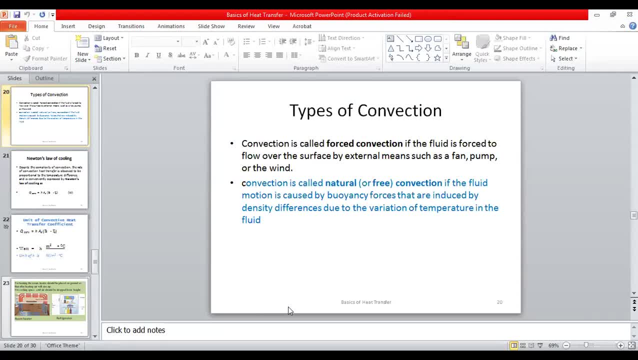 Don't keep the comedy names. And Kiran Malgire, Don't you know your roll number? Don't you know your roll number? Kiran Malgire- Sorry sir, Don't you know your roll number. Don't you know your roll number? 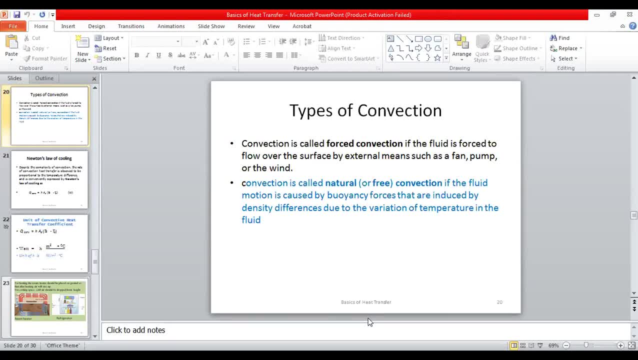 Yes, sir, Then rename yourself. Rename yourself, Okay, I will not tell you one by one to everybody: Naman Kathmandu. Rename yourself. Write down your roll number. Okay. There are two types of convictions: Fourth conviction and free conviction. 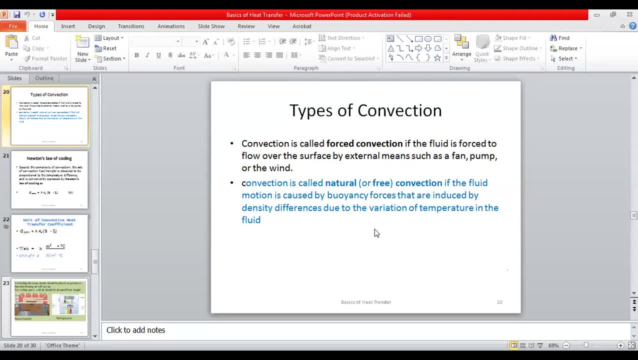 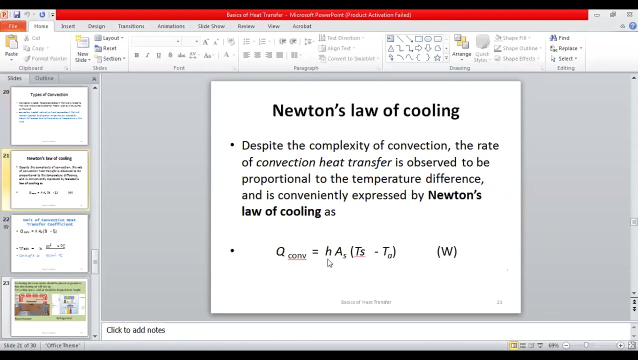 This we have seen yesterday. Free conviction is also called as a natural conviction. Okay, Participants, Yes sir, Yes sir, Okay, Okay, Now we will move to the next one. This formula for convection, i think you have seen q. convection is equal to h as ts minus ta. 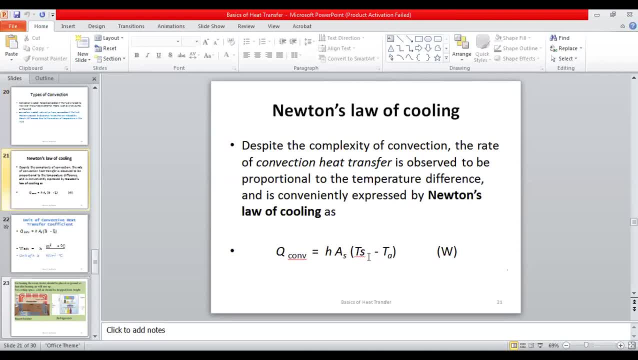 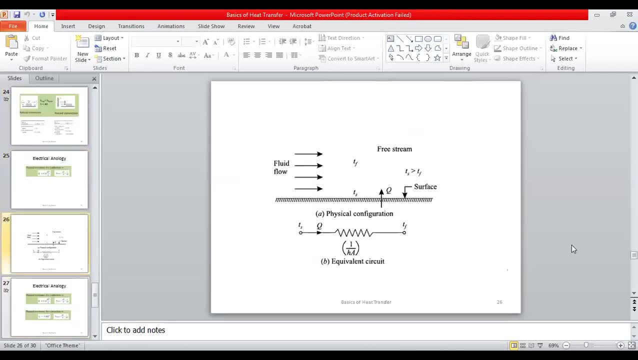 okay, where this is the surface temperature and this is the atmospheric temperature. this you can see here on the screen. see, this is a heat transfer. if this is the surface and heat is being transferred from this surface, and if the temperature temperature of this surface is ts and normally, 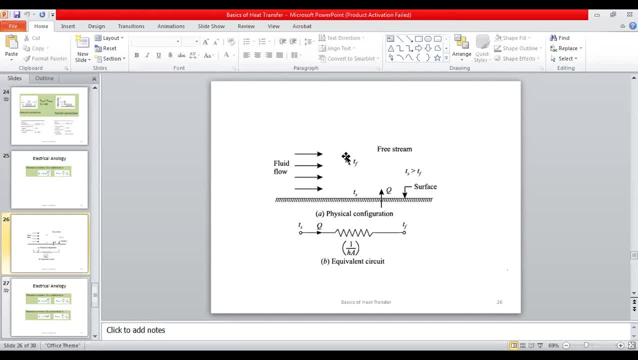 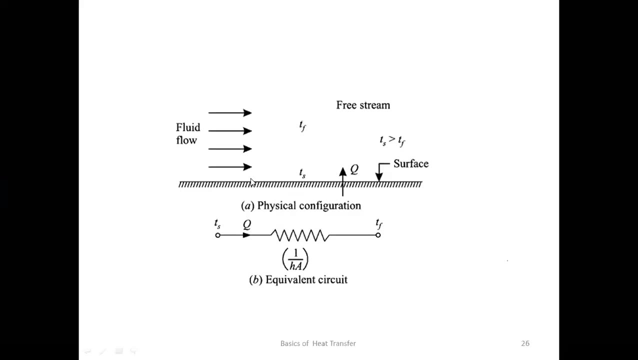 in convection, the air temperature or liquid temperature. both are fluid. hence the fluid temperature is denoted as tf- okay, good temperatures will be denoted by tf and surface temperature will be denoted by ts. okay, ts minus tf. if the ts is greater than tf, surface temperature is greater. 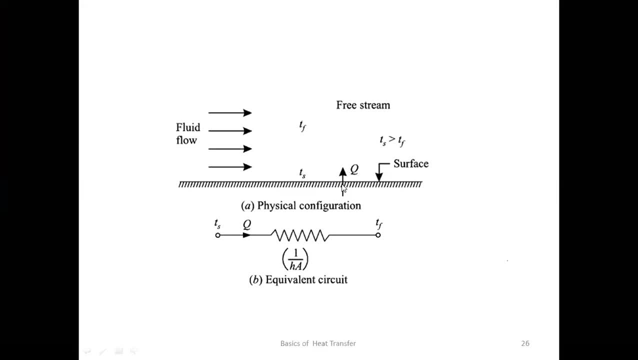 than fluid temperature, then the q will be, or it will transfer from surface to fuel. and if don't play with screen or don't touch the screen, don't touch the screen if ts is sorry, if tf is, if tf is greater than ts, then the heat will transfer from fluid to surface. okay. 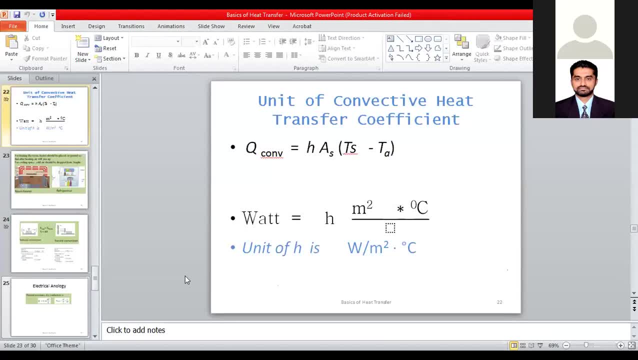 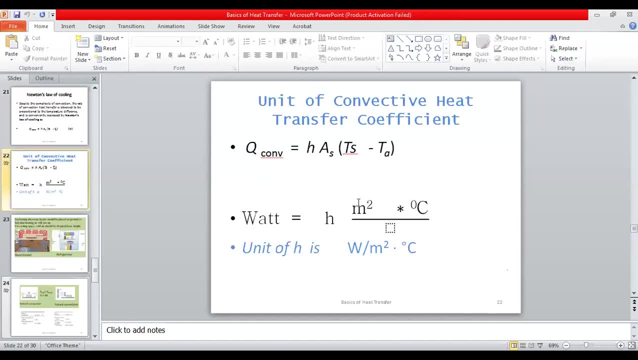 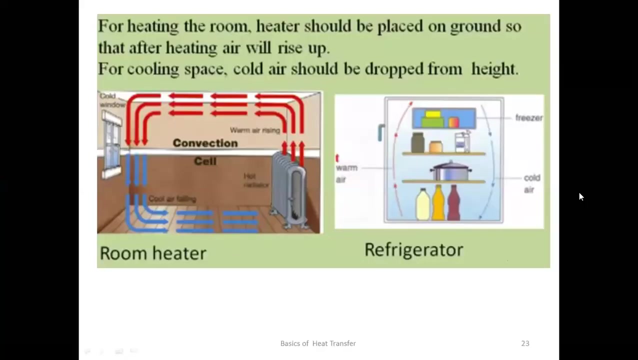 now, i think, unit of h- h. what is the h? h is called convective heat transfer coefficient. okay, what is h? h is called convective heat transfer coefficient. then, unit of h is watt per meter square per degree centigrade. okay, now next thing, and this: i will make a slide show for this, because this is the um. 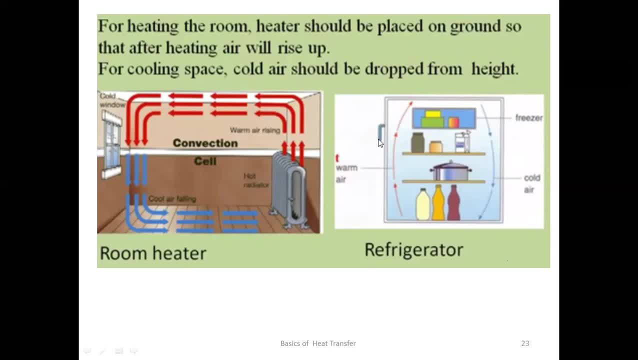 example of convection. first of all, this is what. what you can see. this is the refrigerator: refrigerator, written there, but at least you should able to read that this is the refrigerator and this is the what this is. the red lines are there and these are the blue lines. 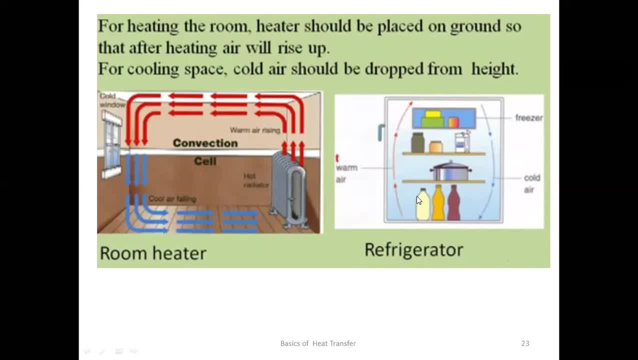 okay, here the this is the warm air or hot air and this is the cold air, okay, you can see, in refrigerator the freezer is always kept at the top side of the freeze because once the cold air- okay- rejects the heat, when the cold air, when the air- sorry, when the air rejects the 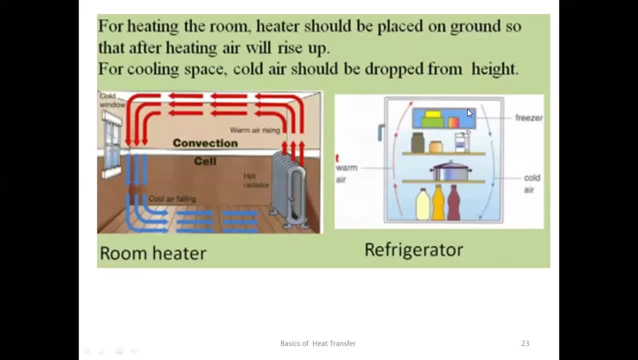 the heat it becomes cold. and when it becomes cold it's density will be larger or more, and because of that it will be means the high density air molecules will go to the bottom side and the low density warm molecule means, after absorbing heat from this surface, these objects okay, whatever. 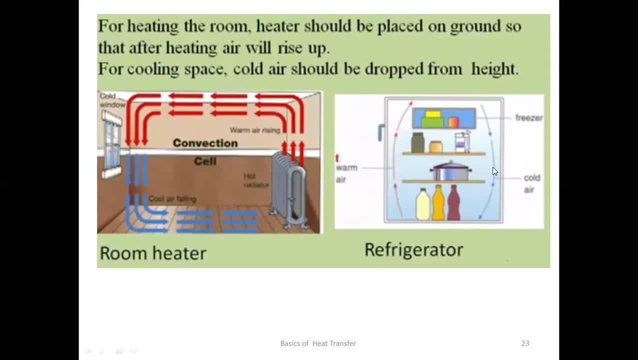 objects are kept, they will reject their heat and these are used to absorb the heat of the surface, their heat in the they will. this air will become warm and again they will go lifted on toward the freezer. again freezer will take the heat from them and their density increases and again they will go to the bottom side in this way, 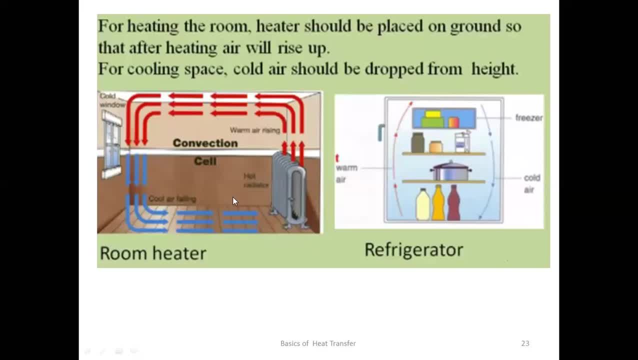 the circulation continues in the refrigerator. now, this is the room heater. this is not used in our countries. this is not only use cold countries, cold countries just like Greenland, Iceland, England, where the room heater is there okay. the hot radiator, okay. this is the hot radiator is there okay. 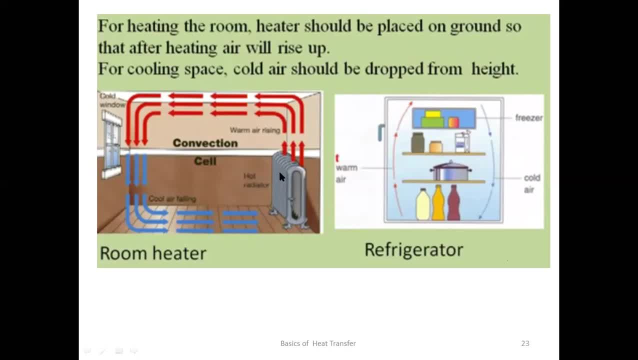 you and see what are these? warm air rising. okay, warm air is rising, and students naman kathmandu. don't you have your own number? please rename your students. please rename your students, please rename your text. say it: " who is this? bhakti ki shakti kone. 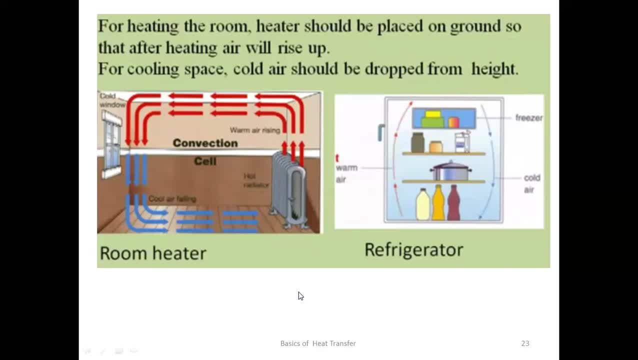 who is this? rename yourself, otherwise your attendance will not be considered. you will be considered absent. who is this? bhakti ki shakti. you exit and rename yourself, otherwise I will remove you from the this meeting. ok, I am removing you now. See, this is the room heater. 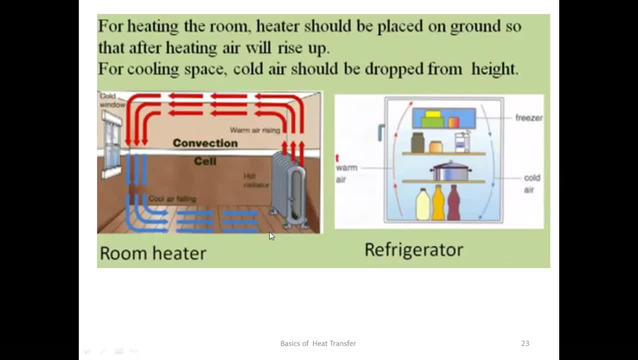 ok, here hot radiator is kept here and See what is written here. for heating the room, the heat so that after heating air will rise up. okay, for cooling space, cold air should be dropped from height. okay, see, if the room is there and radiator is kept there, and 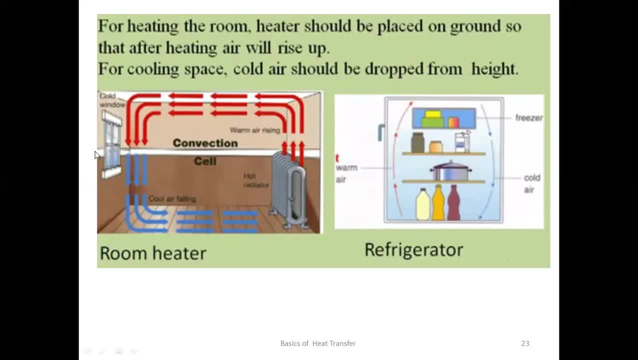 from here. when the cold air, cold air comes from here, cold window when cold air there come, as cold air is having high density, cold air is having high density- it will go to the bottom side and it will take means, it take the heat from radiator and after that the density. 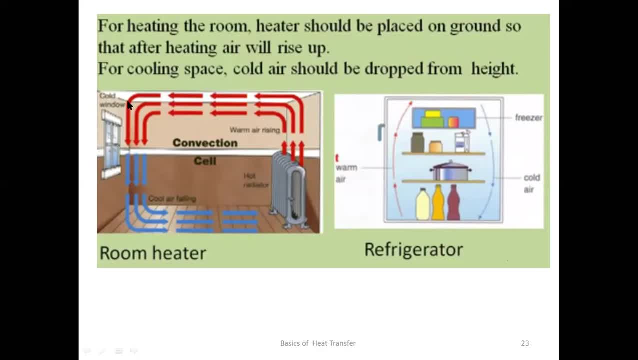 of it drops and again it will go to the means top side. here you can keep ducts also for supplying the hot air to the top of the radiator, to the different corners of the room. here it is not shown but you can design here ducks to the suppose. you can design one room there may be. in cold countries there may be one. 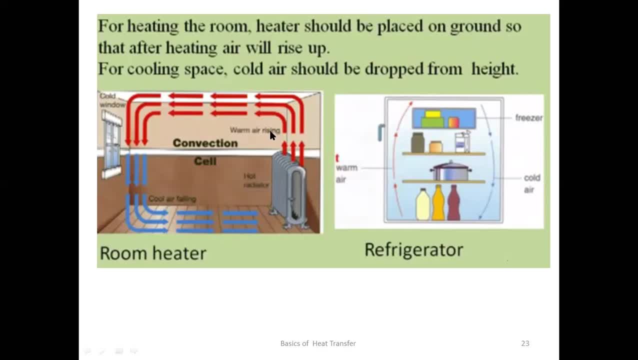 central room will be there, where the heating arrangement will be there, and from that room, the ducks to the different parts of the different section of the room, hello. so ducks to the all of you mute yourself, all of you, mute yourself, all of you mute yourself. okay, see, let's see. 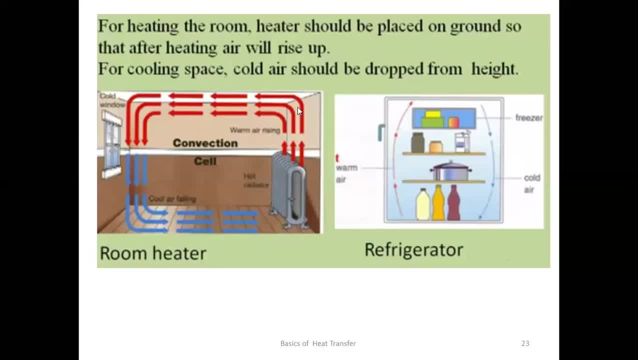 okay, the ducks to the different sections of the house. maybe arrangement will may be made and that warm air is supplied to the house. okay, this may be the arrangement. okay, you are also. i haven't also seen you are. i think you might not have also seen the arrangement there, but this can be there. okay, now next. 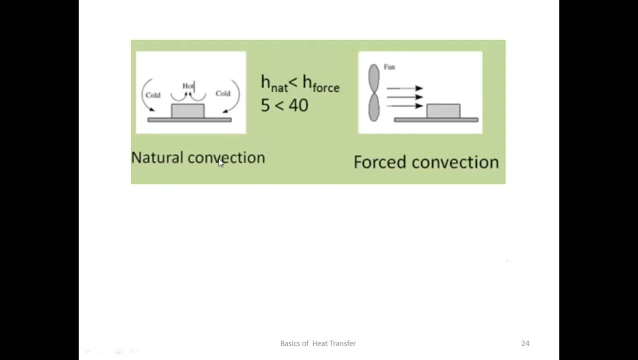 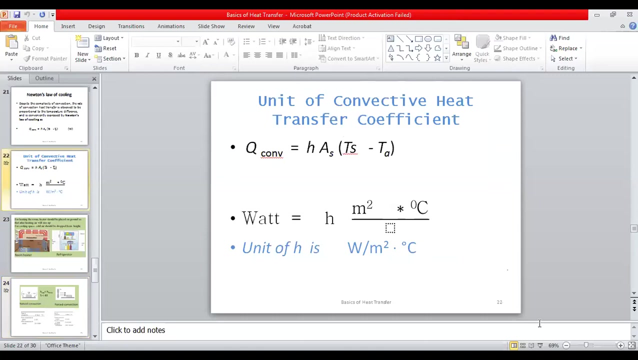 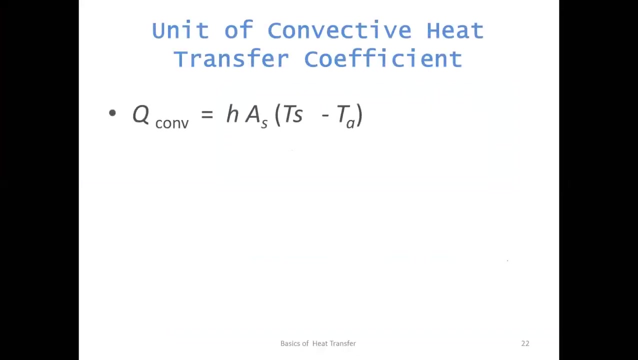 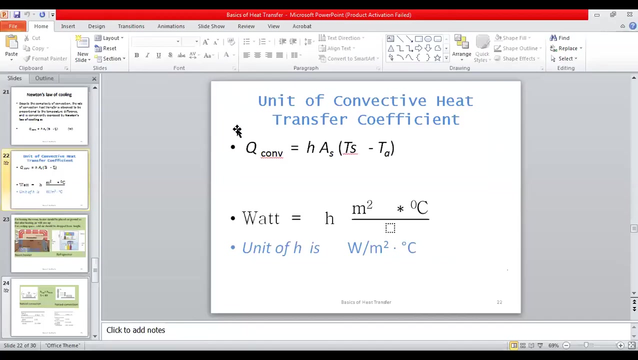 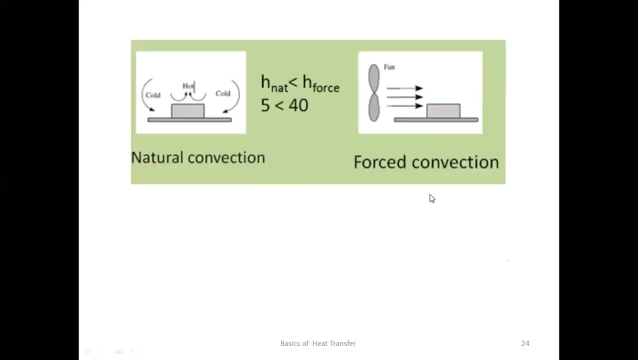 see here: a d 對 a, B A B, again B A B, C A B. the value of h will be different for force convection. the value of h will be different. that we will see now. see here. see natural convection. all of you know this is a natural convection. there is not. 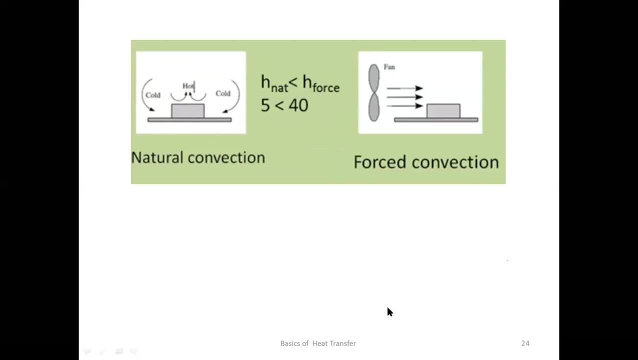 fan is not used here, okay, as fan is not there, hence it is a natural convection. no external power is there and this is the force convection. external power is used. hence see difference in h value: h for natural convection and h for force convection. okay, can you read that? 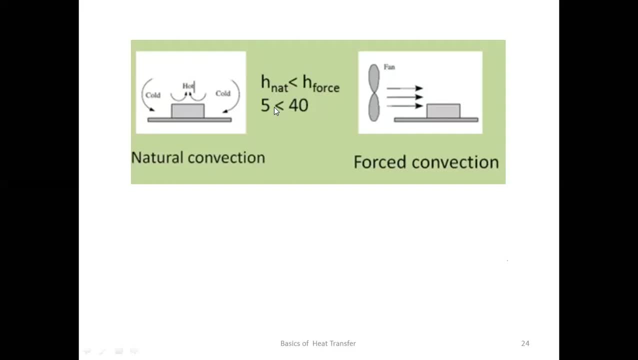 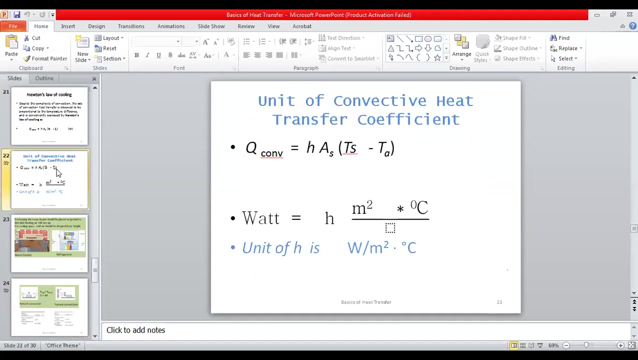 can you read that h for natural convection is 5 and h for force convection is 40. okay, 5 watt per meter square. okay, meter square. kelvin meter square in thermal conductivity: its unit is meter. okay, see unit. what is the unit? watt per meter square, degree centigrade, but here: 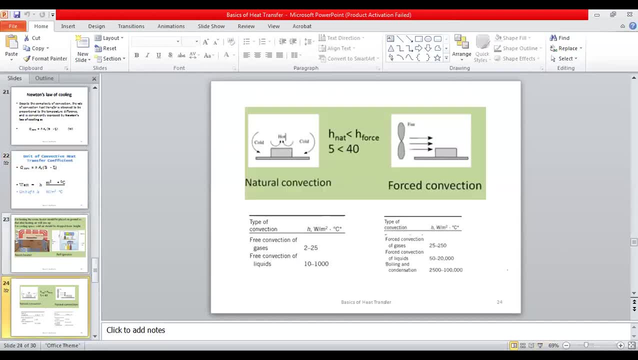 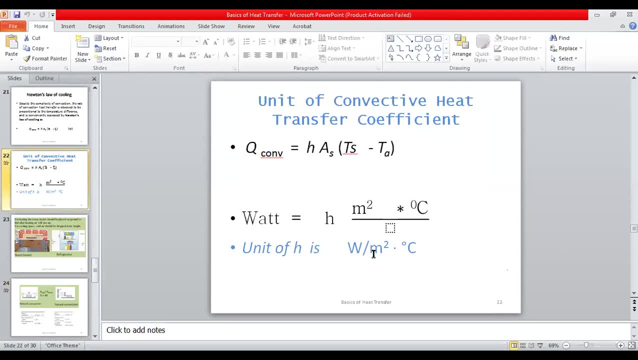 watt per meter square, degree centigrade. but in thermal conductivity there was watt per meter only. this is the difference. there is a difference in watt per meter per degree centigrade and in h watt per meter square, only square term. is there? okay, that remember, you have to remember the 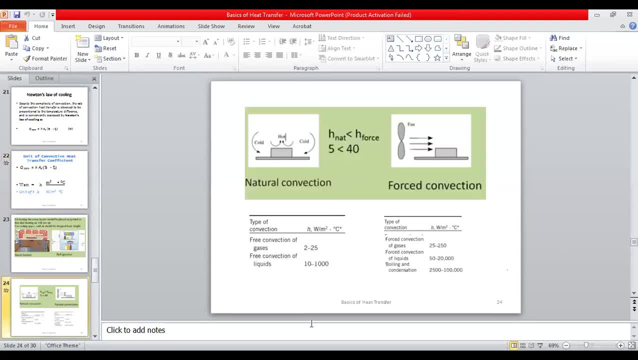 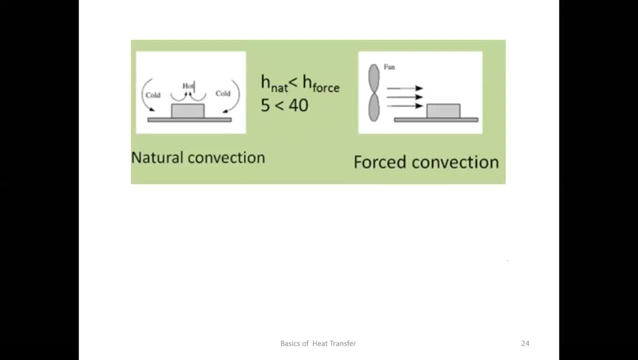 unit also. okay, in future, you will not means forget the unit. also, we have this experience at the time of oral: no one remembers the units. okay, hence i am again repeating this thing. why? because this is the basic part. this is important from theory as well as to understand. 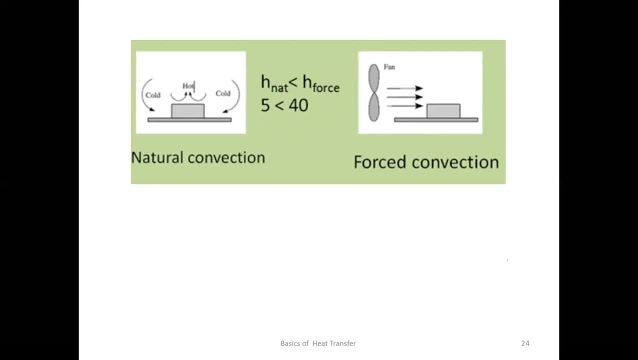 but that is what we will see in the next lecture. okay, see you in the next lecture. bye, bye. this overall point of view, Okay, And also for throughout your life: whenever you face the interview, the questions will be asked to you, definitely, Okay, Now see the next part: See, sorry. 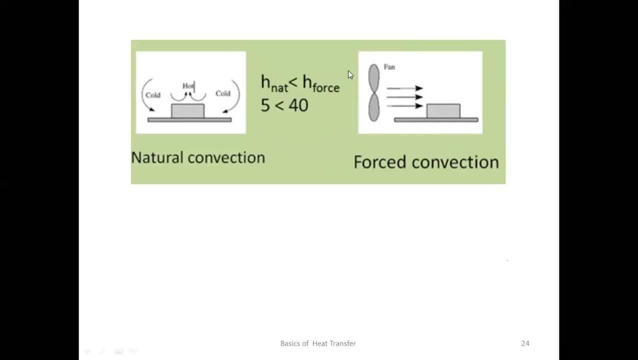 this I forgot. as for natural convection is for you and at the same time. now see here in both the cases. here fluid is used as air also, here is also air, but as fan is used, the air velocity will increase. objects are same now see in thermal conductivity. 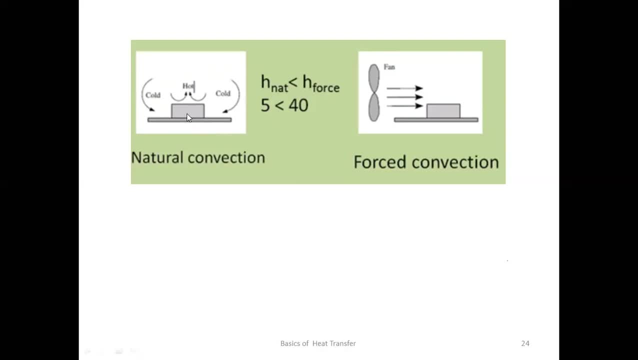 if conduction is there, then K value will be same for both the cases. in thermal conductivity we are not bothered about whether there is a fan is used or not. But here, if fan is used, the value of H will be different for the same size area. 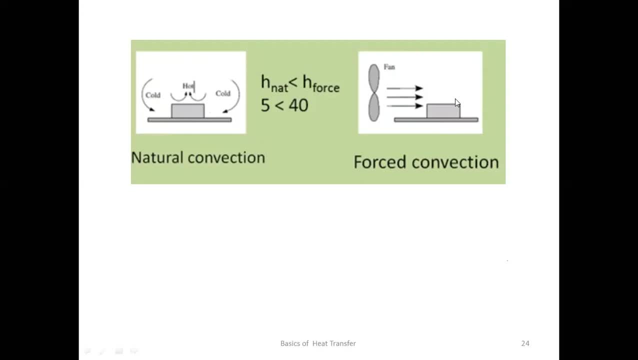 See both. in both the figures the object is having same area, but here and in both the cases air is used, but because of use of fan the value of convective heat transfer coefficient is increasing. Okay, more 40 as compared to final. see the difference how much. 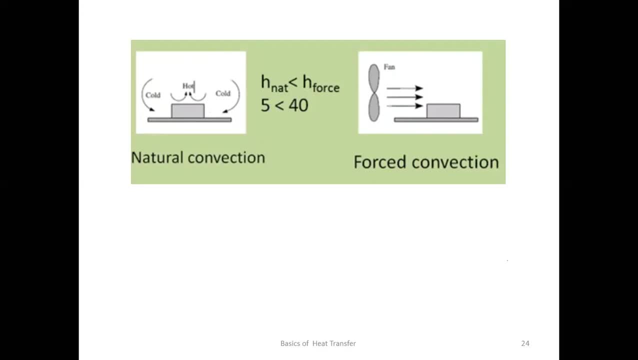 difference is there, Okay, Hence the fire. calculating or finding out H value practically is much more difficult. Okay, when you see the practicals, you means all aspects you have to take into consideration, just like temperature of air, temperature of surface fluid, velocity of air and thermal conductivity of air. 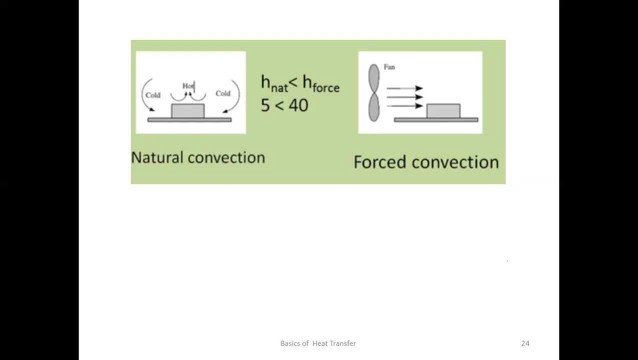 specific heat of air and various things are there. at the time of practical, you will get- and not always we will be getting- the perfect value of H. We have to do some assumptions and on the basis of that we are finding H value. Okay, this is very difficult to find. Now, you see the 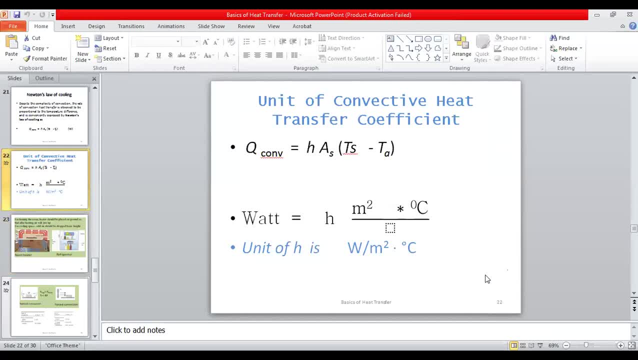 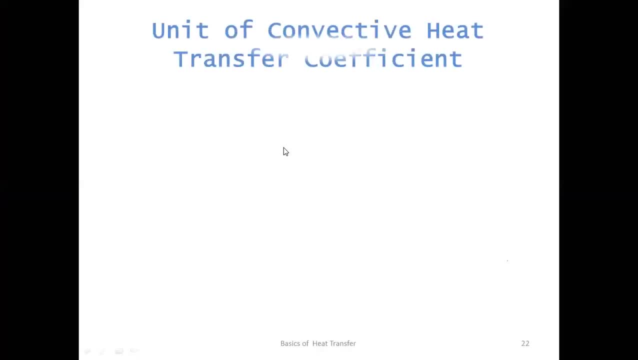 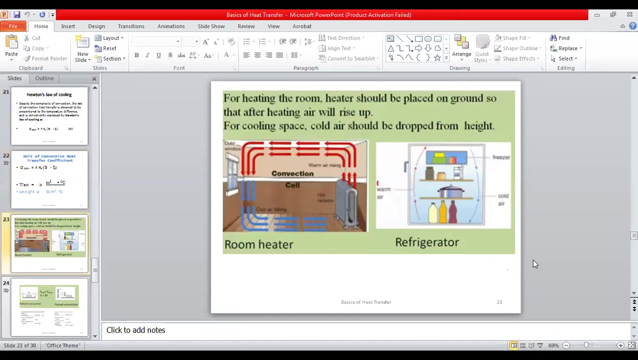 formula is very simple. This formula is very simple, But they are: finding the H value is not that easy. Okay, Finding the H value is not that easier. Okay, Remember this thing. In future, you will face this problem. Okay, the convection is much more difficult as compared to. 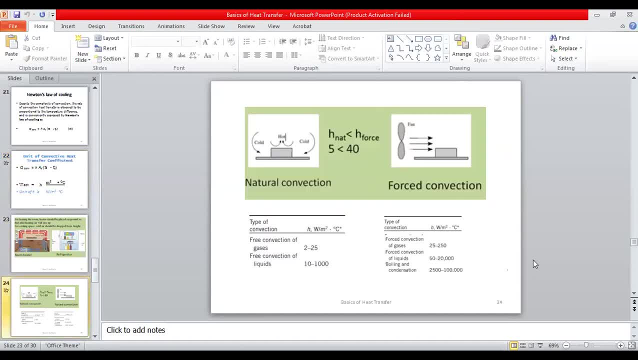 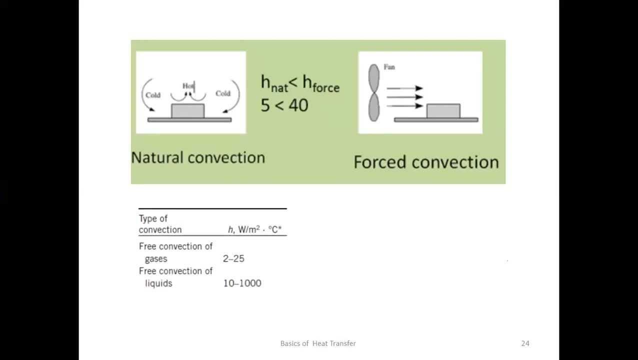 conduction and radiation. Now see here again and again. I am going to that slide because these are very, very important things. again and again. why I am doing this? because once the mathematical derivation comes, there is not any meaning. you have to just buy a hat, that and. 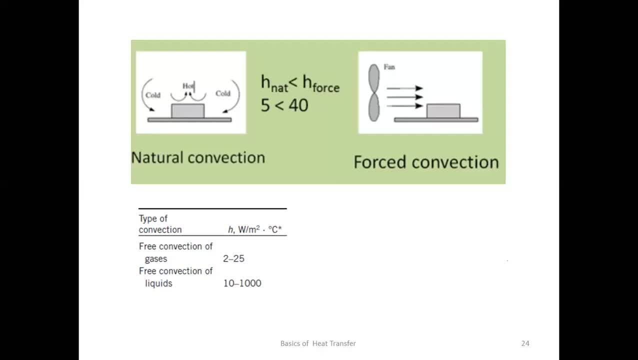 write in the exam, But then these concepts are understood at any time. you can do the answer or write any exam. Hence I am again and again repeating these things, because this is very, very important thing. Now, see here- This is the table- type of convection: free convection and free convection of gases. 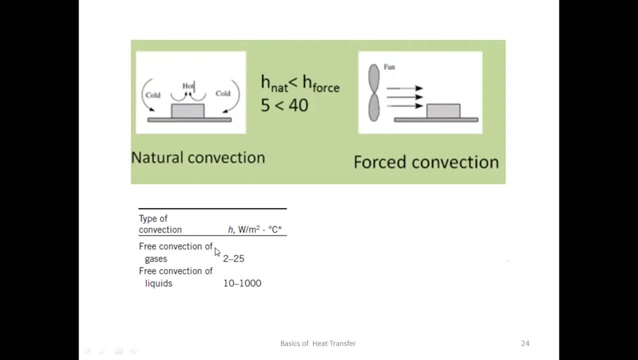 and free convection of liquids. Okay, Now see for gases. the free convection range is from 2 to 25.. Okay, Gas means you can take air. it can be from minimum value can be to the. at the most, maximum value is 25.. If you want to increase the value, 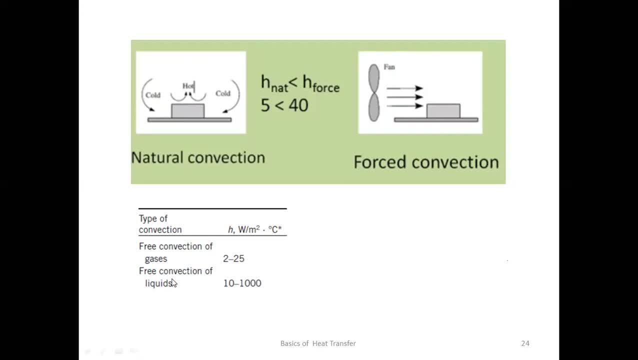 beyond 25, you can't use air, you have to use liquid and that liquid is nothing but water. you can say water Okay means for water. you can achieve the value from 10 to 1000.. We see how much. 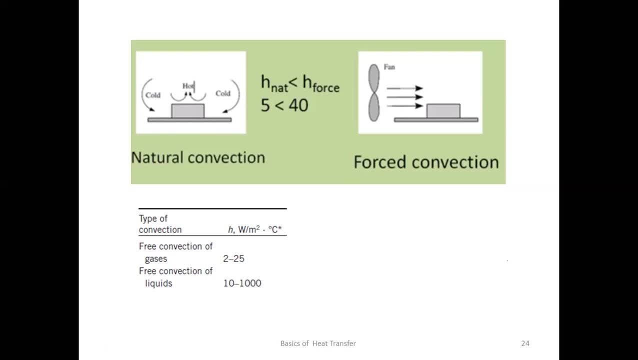 fast heat transfer rate will be there when you are using the water. all of means, if you want to pull something, if you keep that thing in normal air, see how much time is required- is the same thing you keep in a normal water, then how much part that thing will be cooled down. 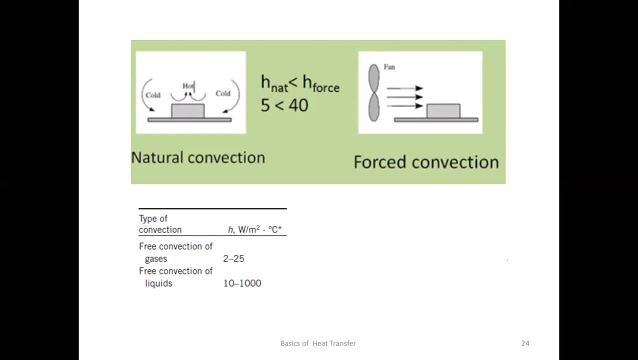 Okay, this is the day-to-day life. experience is there: when you use the liquid, the value of H increases, hence Q increases, and that object get cooled early. Okay Now. next see type of convection and here force convection. now see for same thing if gases are used, here both the 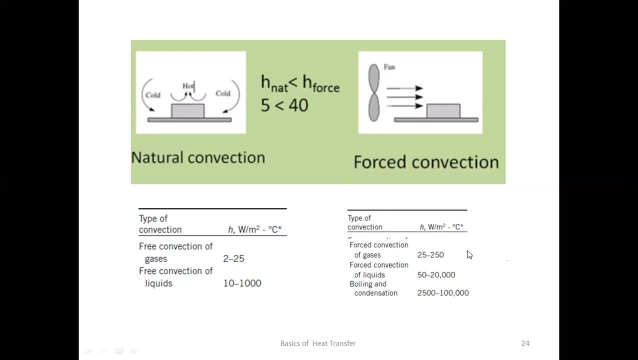 cases you can see. compare: here gases are used, here same means, here also air is used. here also air is used, but here force convection is there. because of the force convection the H value. see tremendous increase in H value From 25 to 250, here 2 to 25, but here there is a tremendous 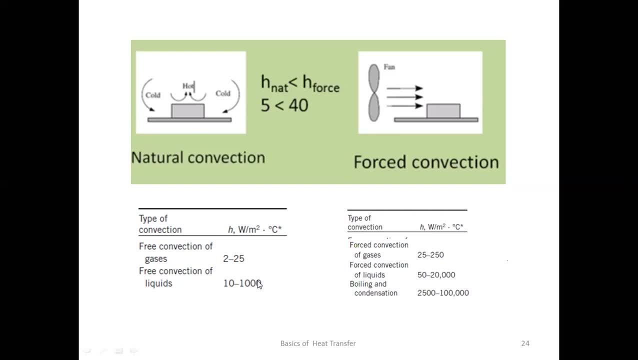 increase in H value and see for the same case here for liquids. here, up to 1000 we can achieve by free convection, but by force convection we can achieve up to 20,000.. Can you imagine this? up to 20,000. I will take the attendance. 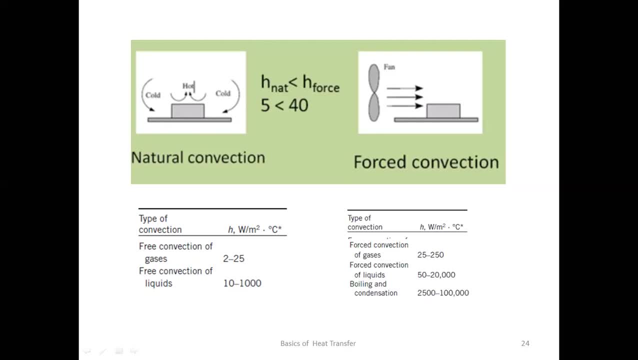 Okay, Print screen. Okay, Now I will not take the attendance after this. only 13 students are there. Okay, and see at the last boiling and condensation, see the value. Can you read maximum value? Anybody can read for me maximum value of H for boiling. 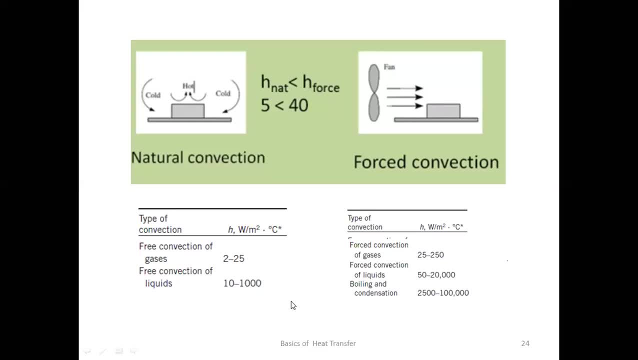 How much is that? Why we read anyone. What is the maximum value of boiling for condensation? Sorry, Maximum value of H for boiling. Anybody from you? I have to just see. Read out for myself. To the one finder. 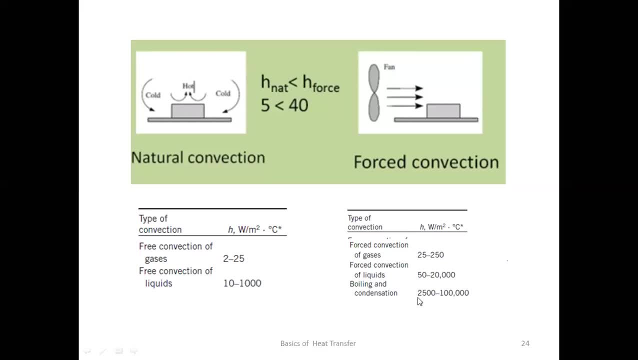 To maximum value, To like one, like when let's see For boiling and condensation The maximum value is 1 lakh. near about 1 lakh means very fast heat transfer rate is there because here the phase transformation is there, from liquid to gas or from liquid to solid. 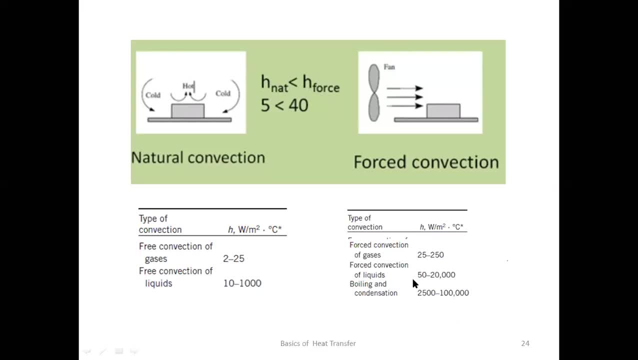 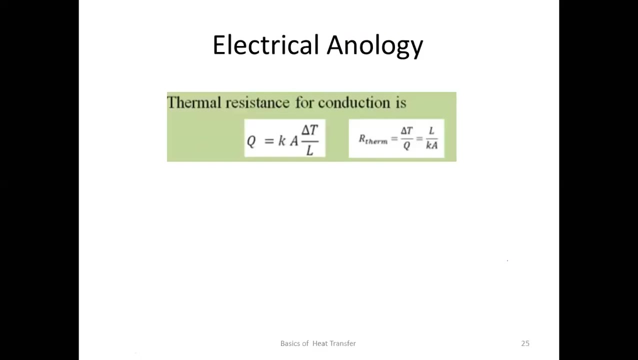 Okay, Hence the Latin heat is comes into picture, Hence the there is a more and more heat transfer and the H value increases. Okay Now, next slide. Now we will see the electrical analogy. Okay, This formula you already seen. Q is equal to K, a Delta T by L. 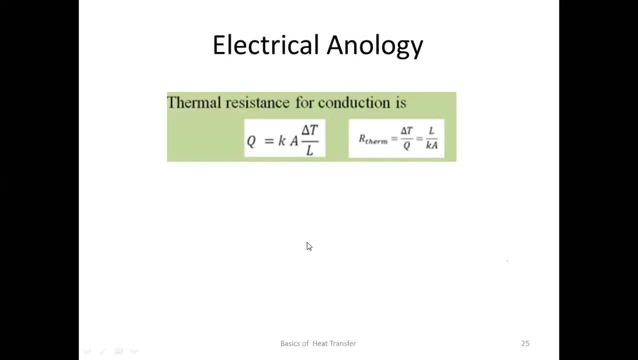 This is for conduction. Now for this, For this R thermal resistance. Okay, The R thermal resistance, Delta T upon Q. Okay, What is the formula of thermal resistance? You know that electrical resistance Formula: Delta V upon I. okay, Voltage difference upon current. similar to that, the thermal resistance. 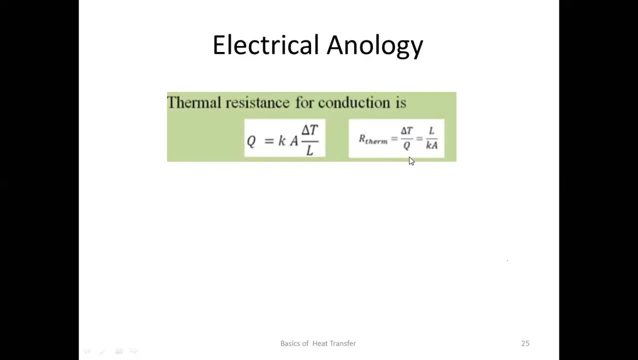 is temperature difference upon heat, because heat is a flowing phenomena, just like a current. is temperature difference upon Q and if you rearrange this, Delta T by Q, L will goes to numerator side, K will go to denominator side. is Delta T upon Q is equal to L by K. 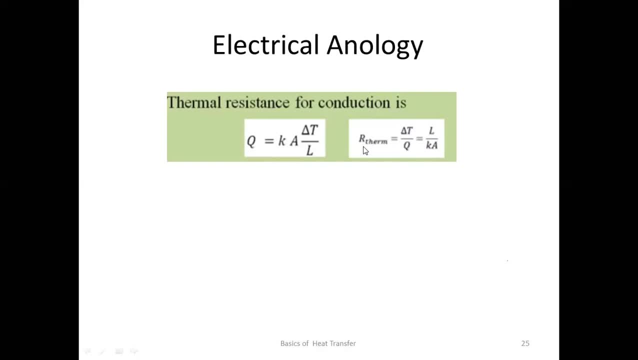 Okay, Either you can use this formula for finding R or this formula for finding R- any formula you can use, and the answer will be same. Okay, Remember these formulas. Okay Now, similar to that. Can you tell me what will be the value of thermal resistance for convection? 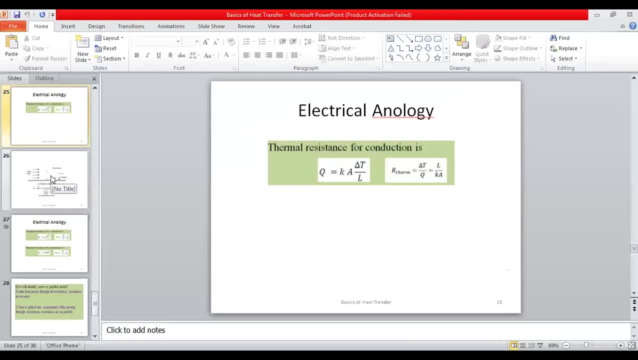 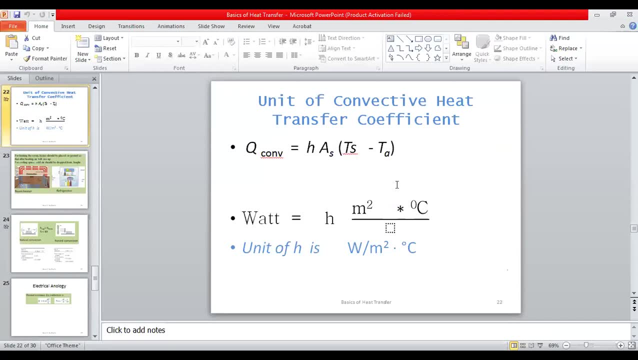 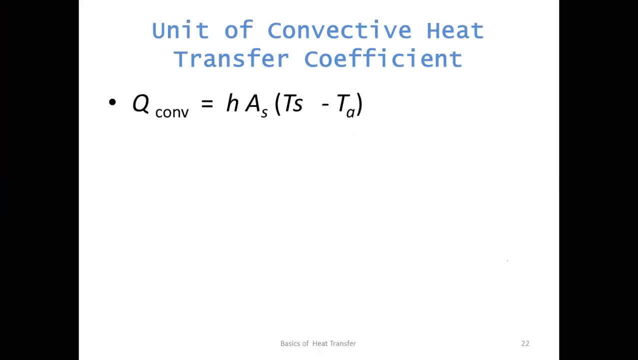 Okay, What will be the value of thermal resistance for convection? This is the formula for convection. Convection formula is: Q is equal to HA. Delta T. Okay, What is the formula for thermal resistance? Delta T upon Q. Okay, All of you. 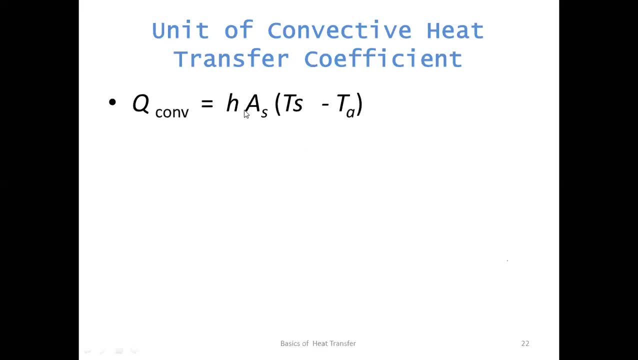 Unmute yourself. Delta T upon Q. Okay, Then if you shift this Q here, then Delta T upon Q will. what will be the? then this will go to on the this side. This is denominator side. Okay, This will go to the denominator side. 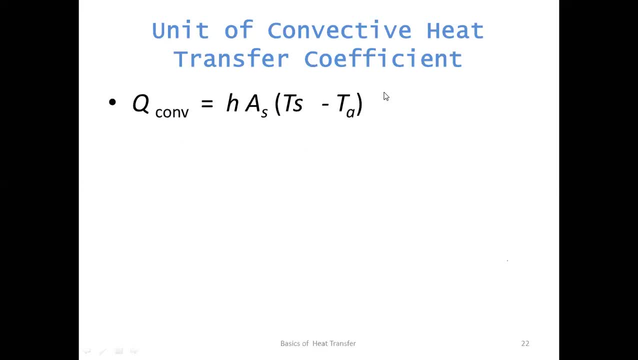 Then what will be the formula for convect? thermal resistance for convection. All of you unmute yourself And tell me the answer: Delta T upon Q. If it comes here, then it will come here to this side. This Q will shift here, then this will go to this side. 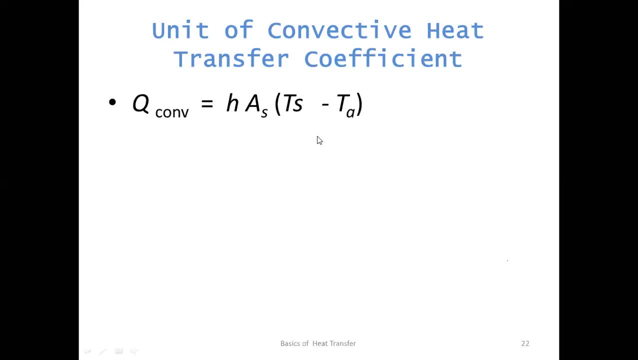 Then what will be the? this Delta T upon Q is nothing but R thermal resistance. This we know. Okay, Okay, Only 10 minutes are remaining. We will continue. Let's continue the lecture. Q convection upon HA is No, no. 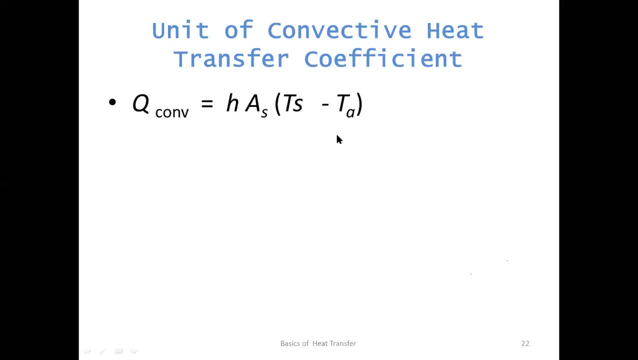 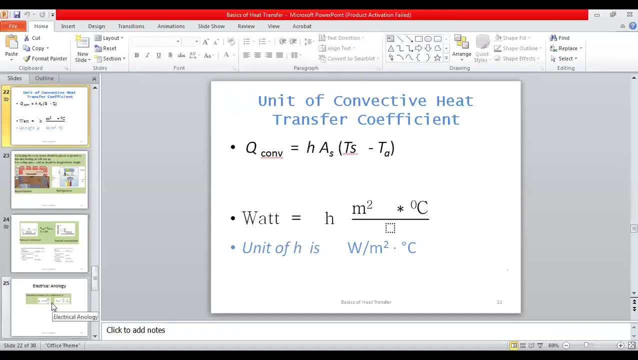 See This. what is the formula for R? Delta T upon A one minute? See this slide. R thermal resistance is Delta T upon Q. Can you see this? Delta T upon Q, Okay, Means Delta T here. Q here means L by K is nothing. 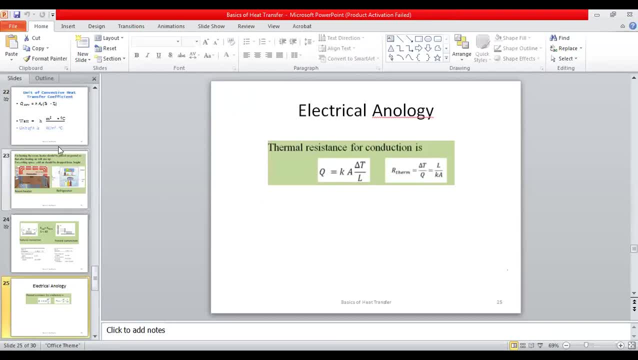 But the R thermal resistance for conduction. Okay, Similar to that. If Delta T upon Q shifts here- Q shift here mean Delta T on numerator side and Q on denominator side- Then this will shift on this side means it will be what will be this on the left side after shifting rearrangement: 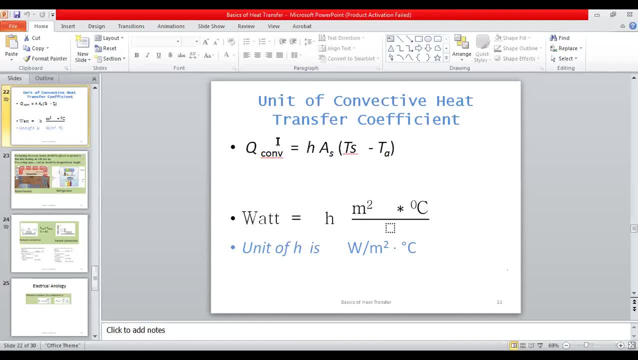 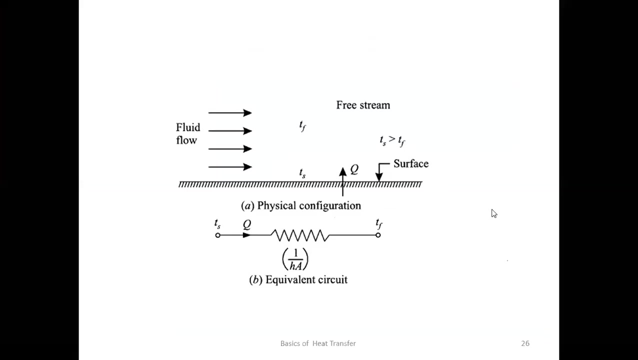 1 upon HAS, 1 upon HAS. Okay, Then that 1 upon HAS is nothing but the thermal resistance for convection. Okay, Okay, sir. See, 1 upon HA is the resistance For conduction Here. L by K. 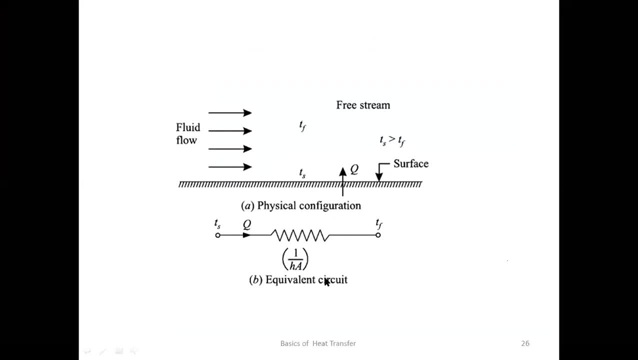 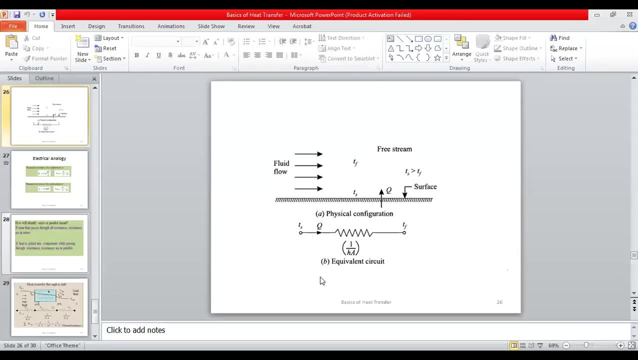 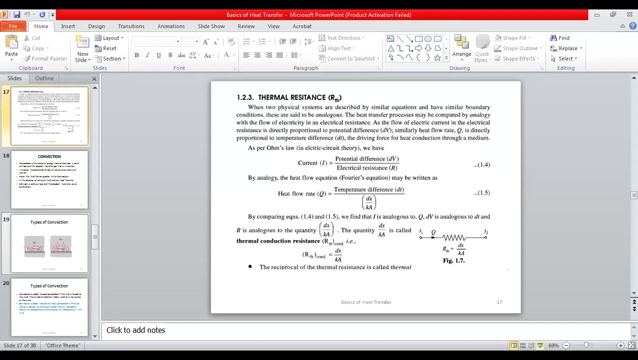 Was there Okay here. L by K was there Okay, but for convection here, 1 by HA- Okay Again, we will go to the conduction. See this figure, See this corner: L by K for conduction. 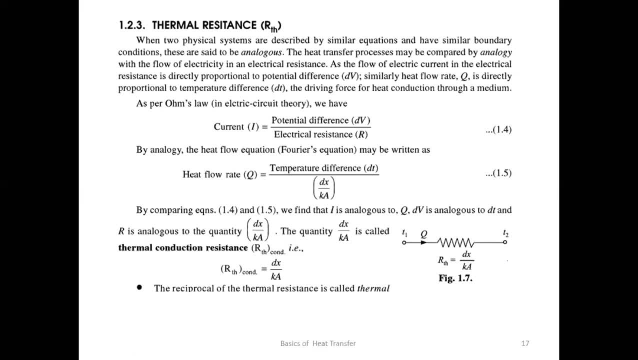 Okay, We are running out of time, But again we are going to join up Because I have to take attendance again. Some students are going: Okay, see L by KA. For conduction: Okay, but for convection, What will happen? 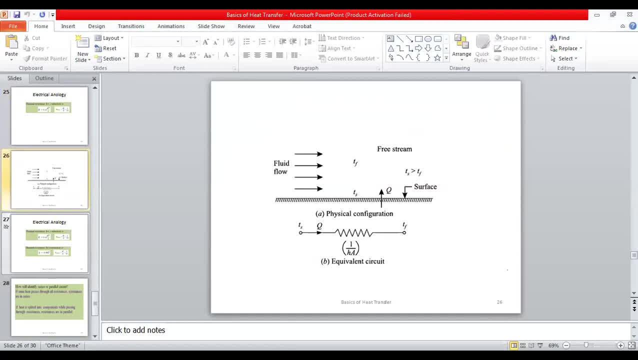 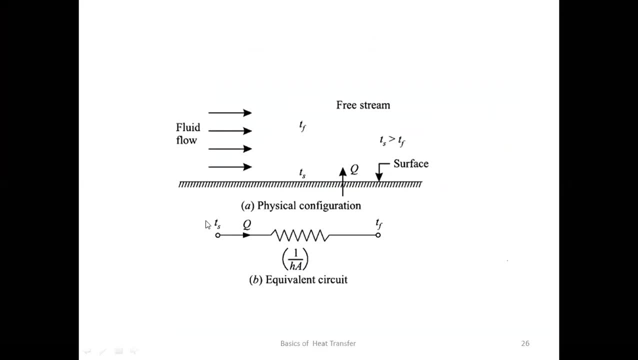 See this: 1 by HA getting these high temperature to low temperature, Because here eic is more, then the F and seat is being transferred from surface still further. Then he could be transferred from surface to next Cancer at the end here away, there on the left side gains high temperature, here low temperature. 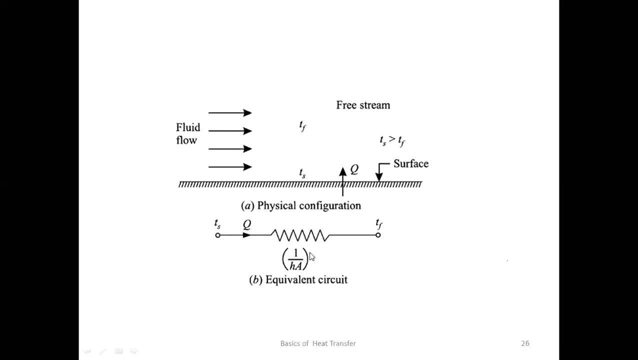 Q is going from high to low and here 1 by HA. Remember four, convection, convection. These are very, very important things. These are used to solve the numericals in future. Okay, Hence you have to buy these things. I am going to share you these PPDs on Moodle, Hence you can refer that. Don't worry about this data. I will share my notes also, books also, and PPDs also, and videos also. Lot of things for you. You have to just study, But you don't study. 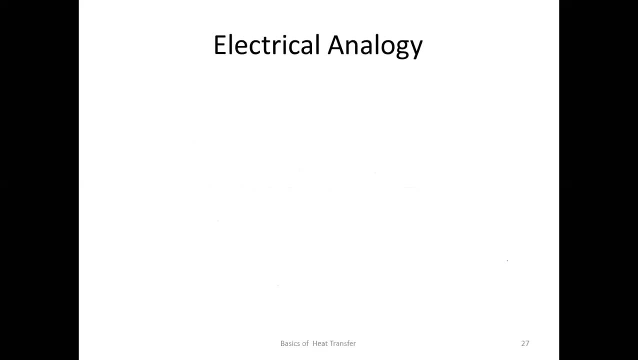 This we know. In this slide, the comparison of thermal resistance, of both the conduction and convection, are done. You can see this. If you can take the screenshot of this slide, you take. Okay, Remember this formula. I will wait here for some time. You can take the. 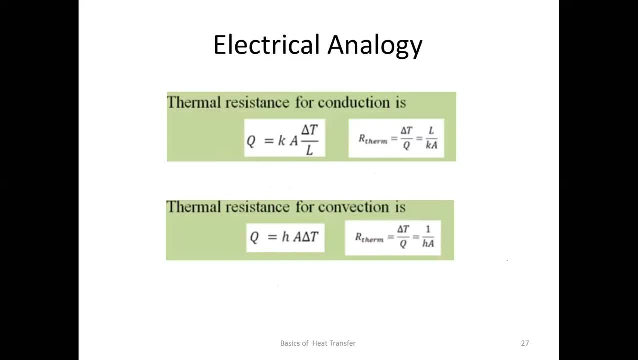 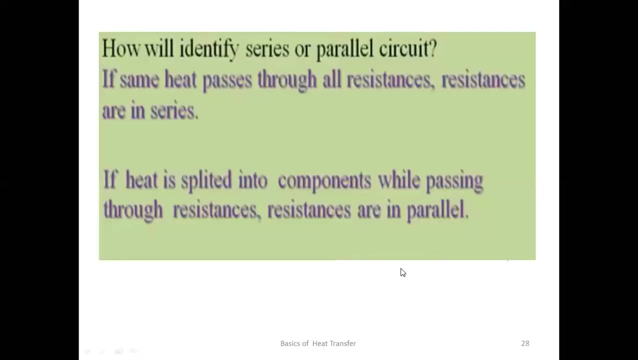 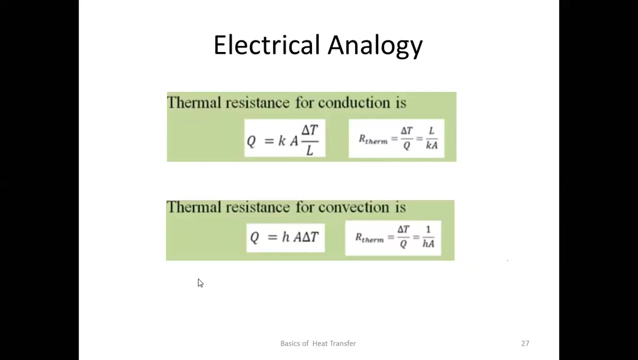 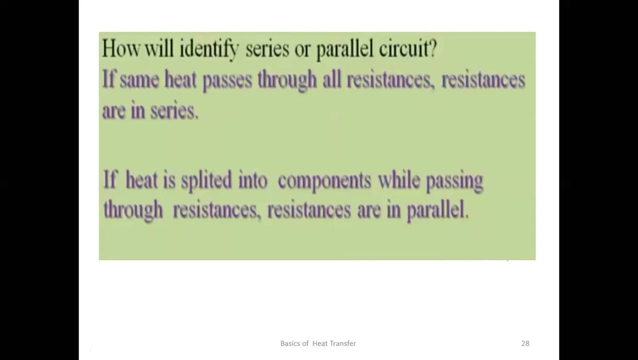 screenshot also: Okay Again, next slide: Okay, How we will identify series or parallel circuits. Okay, Now you have studied series and parallel circuits for electrical circuits, Similarly to that here in heat transfer. also we are studying series and parallel circuits. Now, how to identify. Okay, if Now see what is the series circuit in series. 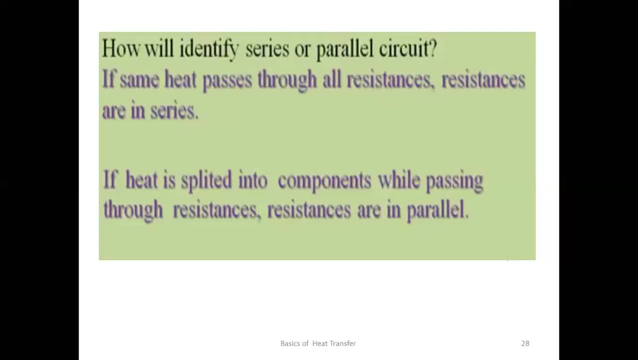 circuit. the same current is flowing In electrical circuits. you have seen that if two resistances are kept in series, then same current is flowing, and if two, what two resistances are kept parallel, then current is divided into two parts, Only the voltage of two resistances. 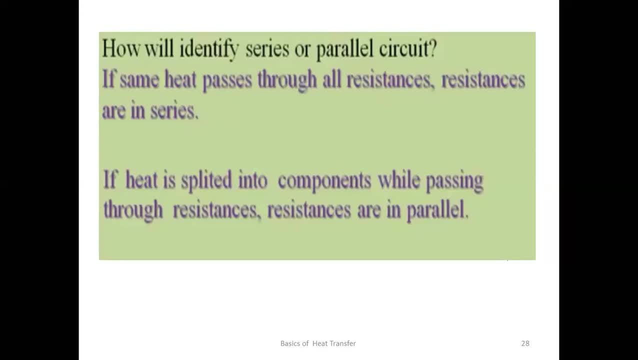 is kept in parallel. Okay, So if there is one power source, then current is kept in parallel. If the power source will be same, okay. similar to that: if the same heat is flowing between the two objects, then they are told to be in series, and if the heat is being divided, that they have to term as. 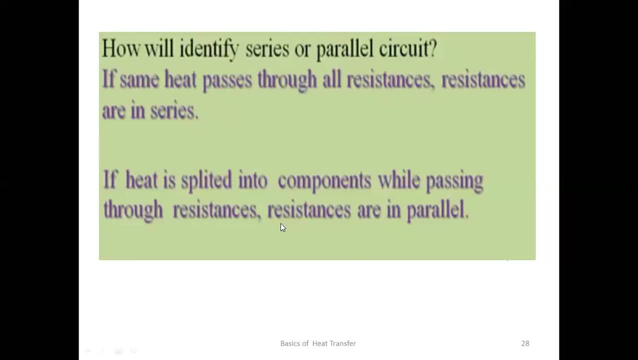 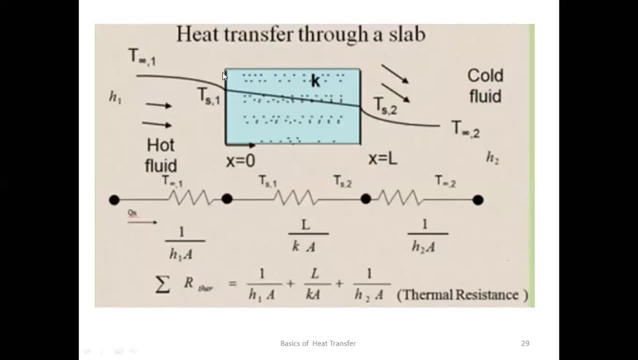 parallel resistances. okay, see here. heat transfer through a slab. now see, this is a wall. you can say: this is a wall from here to here. okay, and inside that wall the hot fluid is there, and outside that wall, cold fluid is there. cold fluid is nothing but air. you can say: 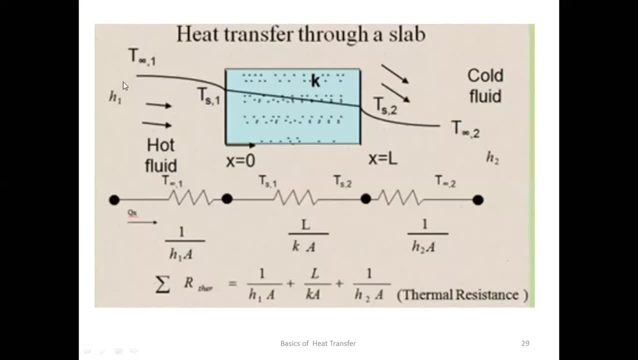 and here water. you can take, okay, water, air, hot fluid and cold fluid. now see here: if heat is transferring from here, this side, if the heat is transferring from this side, this side, left side, hot side, then the same heat will transfer to the cold side after steady state. 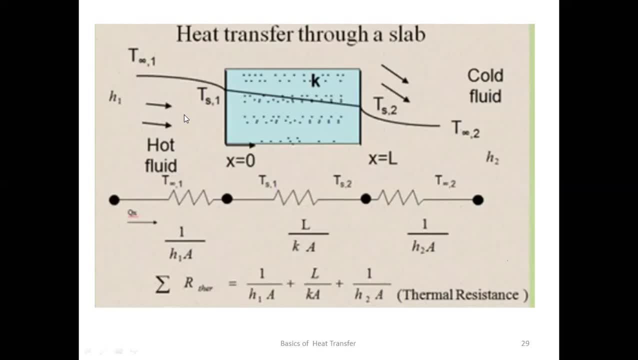 once the steady state is achieved, the same heat is being transferred from hot side to cold side. hence you can say that this is a series arrangement. okay, what this? it is a series arrangement, okay, it is the series arrangement now, here in this arrangement can be shown in a electrical circuit diagram or circuit diagram. you 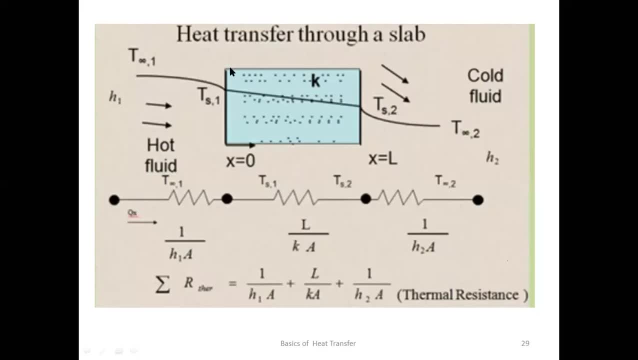 have to draw a circuit diagram for this arrangement. in future, once you solve, when you are going to solve the problem for the given arrangement, you have to draw the equivalent thermal resistances arrangement. ok, here, this is one means. for one fluid. there is one resistance, remember one fluid.